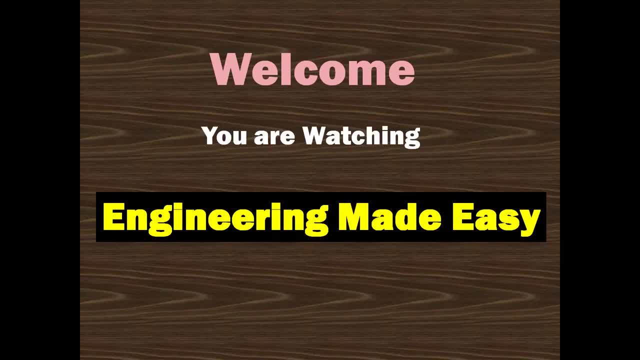 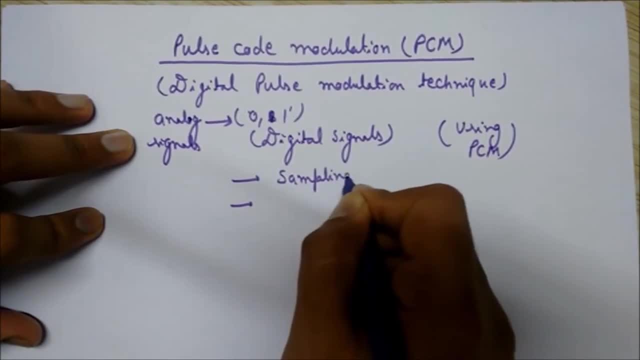 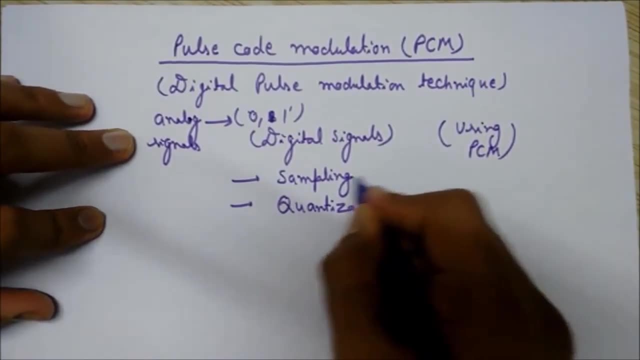 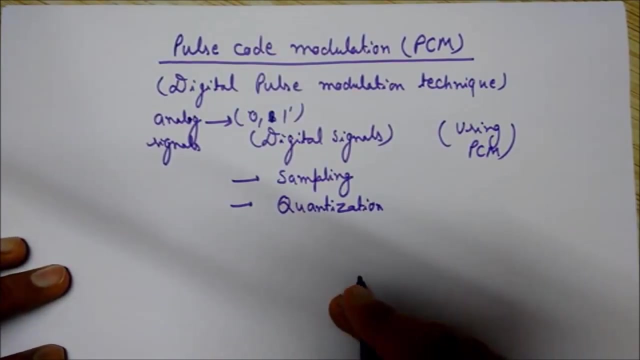 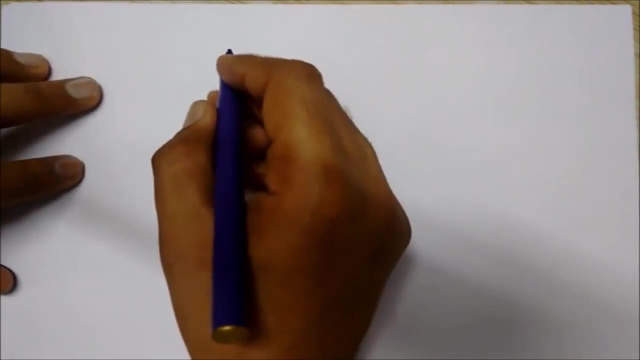 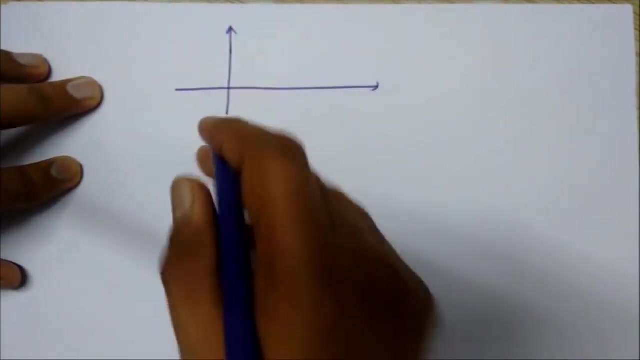 The sampling and the quantization. The sampling is based on the sampling theorem. It cuts the signal into samples using the sampling theorem And in the quantization is at the amplitude level. So to understand it, we need to understand the concept of quantization and sampling. So I will draw a diagram Here. this is a signal. 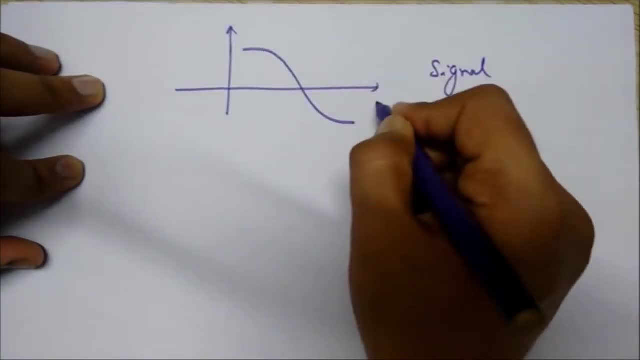 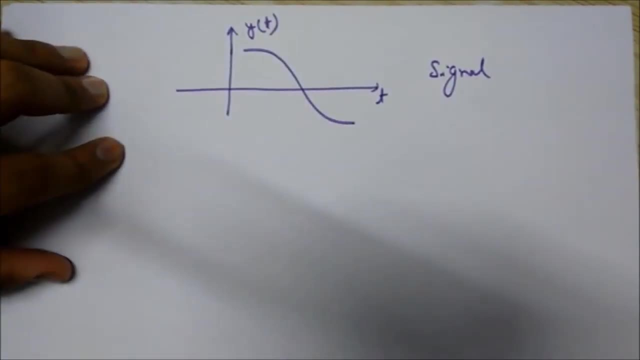 Okay, this is a signal and the time axis Let's call the signal. denote the signal with yt. And here I will sample the signal with the help of sampling theorem. So how does this look like? I am showing it here. 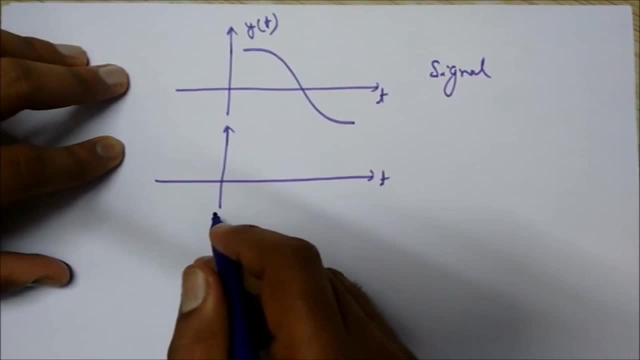 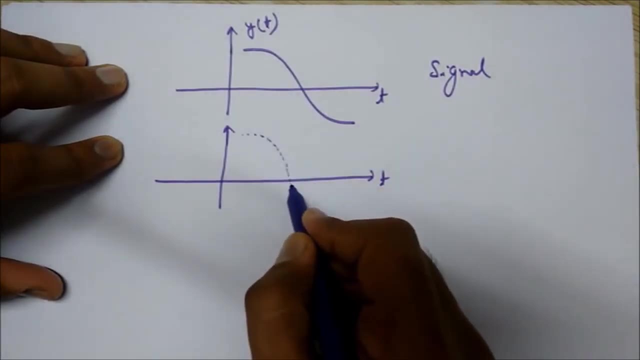 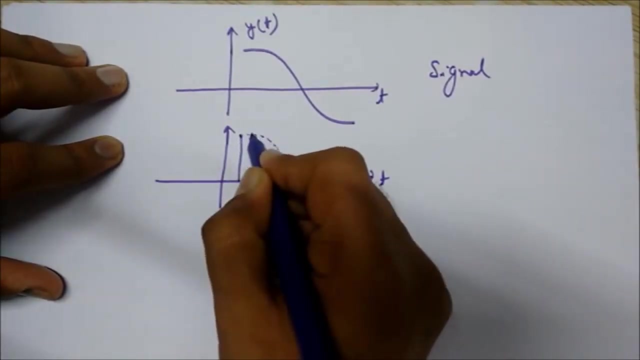 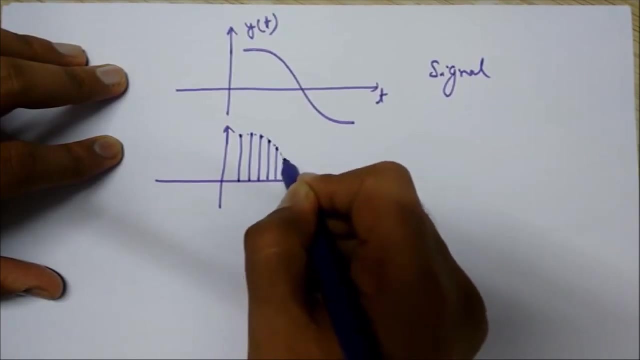 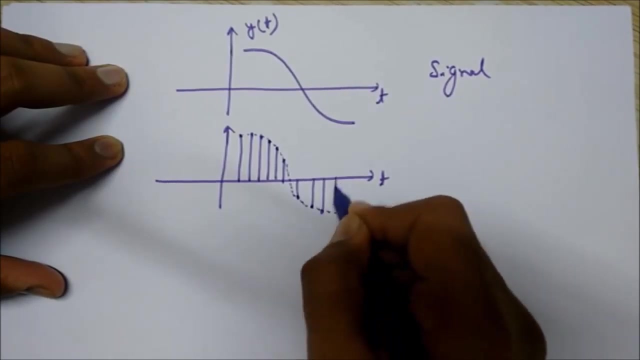 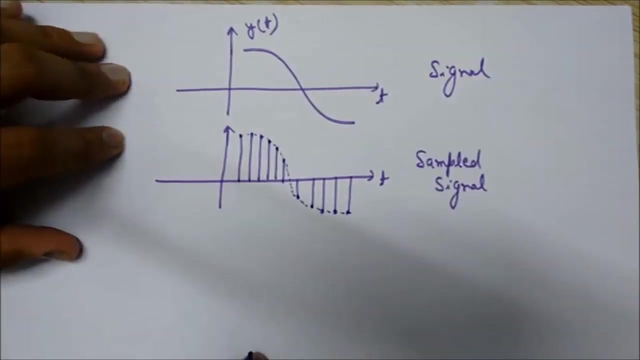 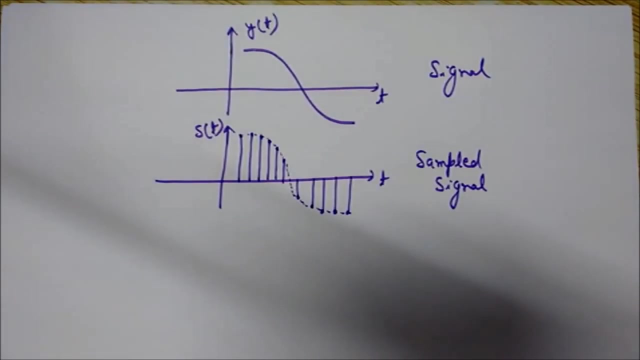 The sample signal is sampled, So this is somewhat of this form. This has been cut horizontally into samples, So this is the sample signal. So this is the sample signal. I am denoting the sample signal with st here. Now we will see the quantization process. 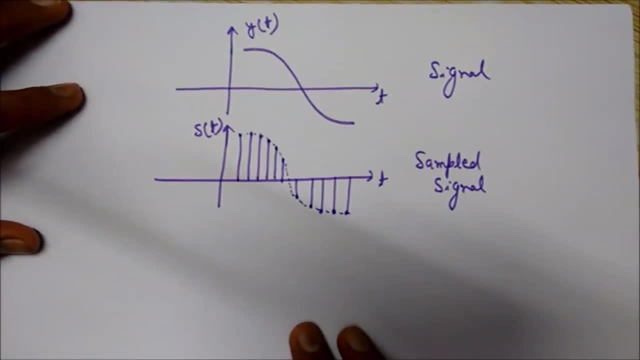 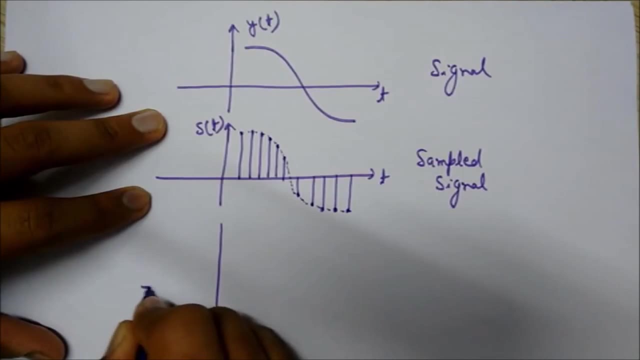 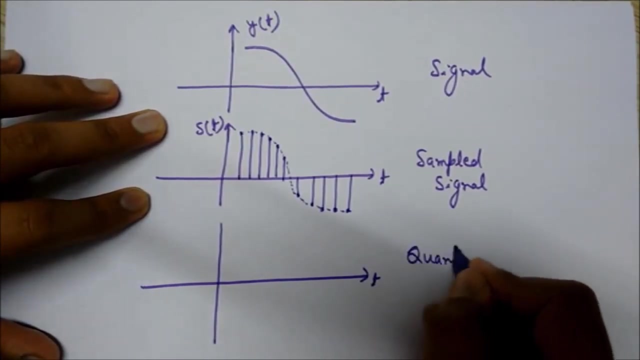 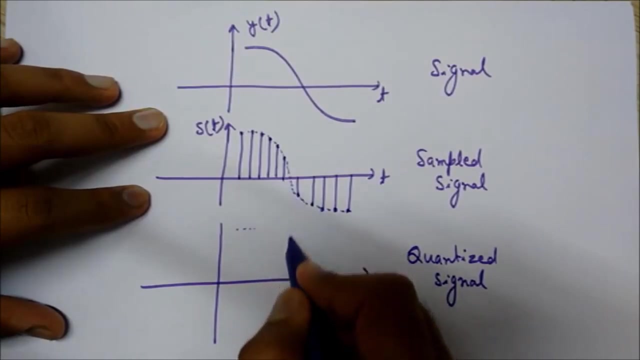 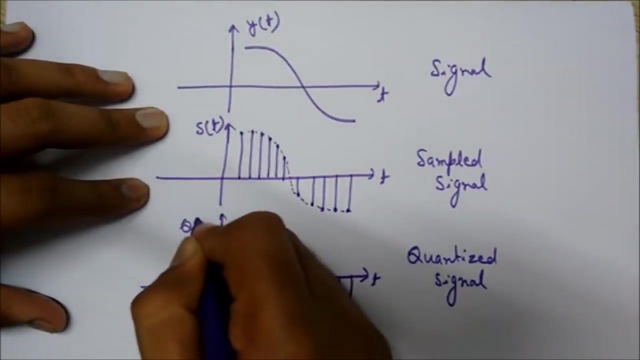 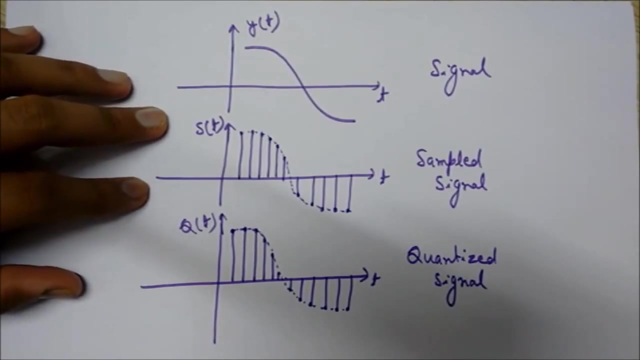 How a quantized signal looks like. So here is the quantized signal. Ok, So let's see here Now if I am denoting it with qt quantized signal. Okay, QT quantized signal. and here is the time axis for quantization. I have already told you the 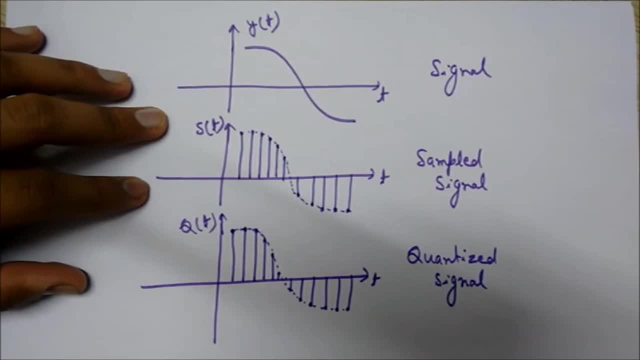 definition and I have explained it earlier. what is quantization? here? we cut this amplitude into number of levels and we try to approximate the value nearest to the. you can say that we try to round off the value of that signal corresponding to that fixed value of level, fixed level value. so 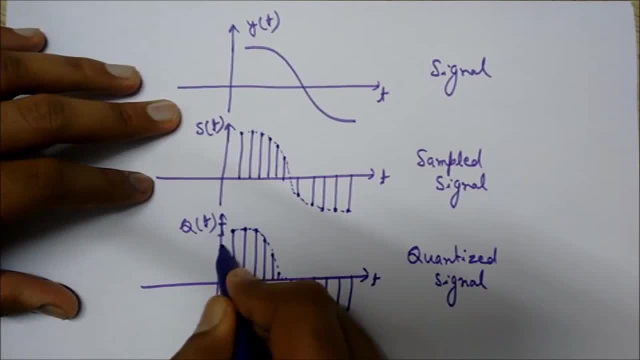 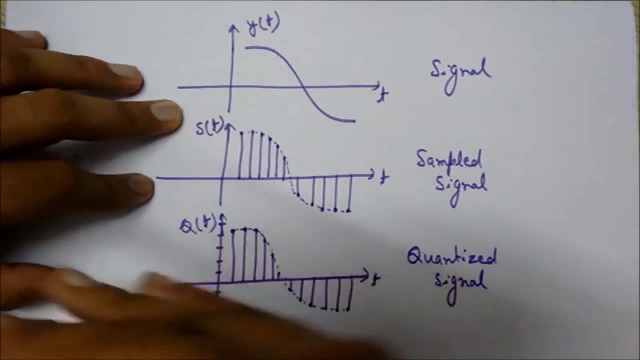 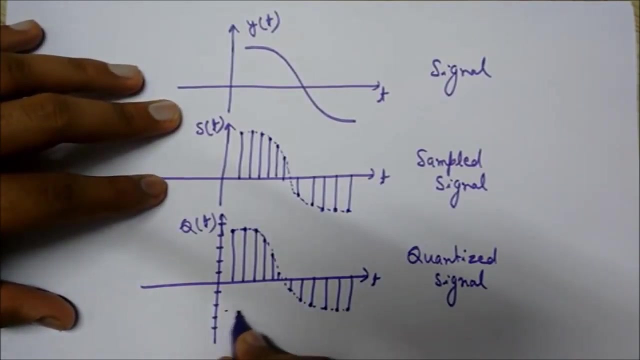 here I am cutting this into some levels: 1, 2, 3, 4, 5, 6, 7, 8, some levels in the help of horizontal lines. let's say that this minimum point is minus QP, and here is the QP. this amplitude is denoted by QP. so if there are L number of 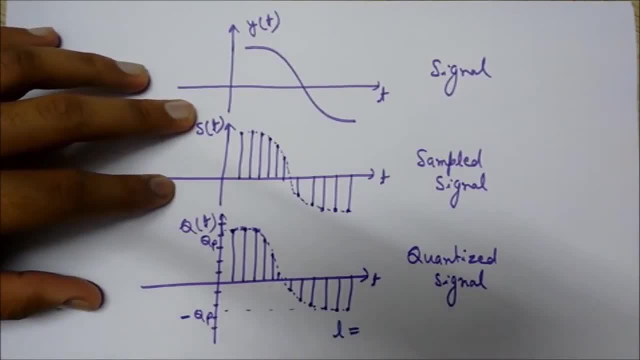 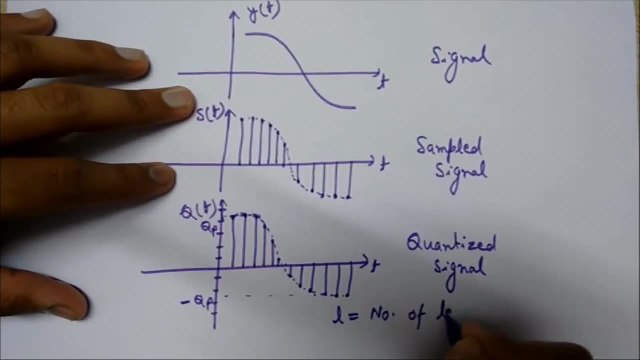 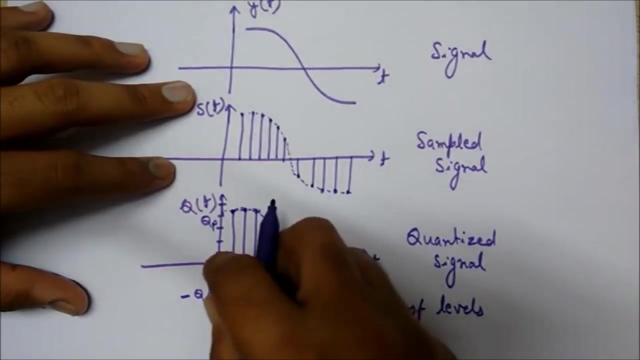 levels, then L. if I'm cutting it into L levels, then L is the number of levels, okay, and two times of QP. you can see this is QP and here it is again the QP, the QP, and QP comes to QP is the. 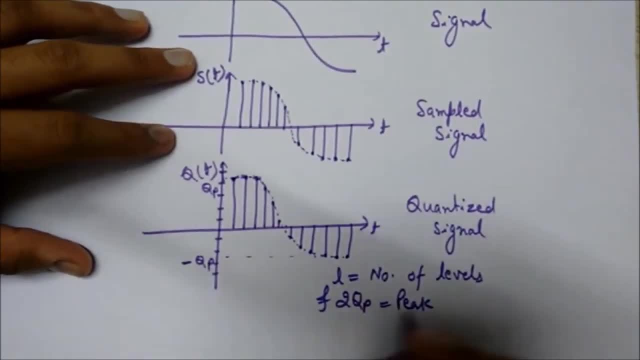 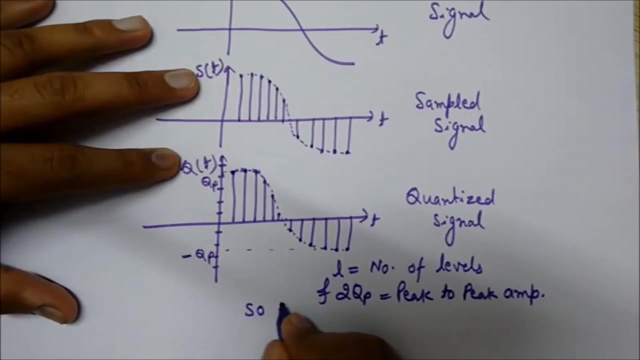 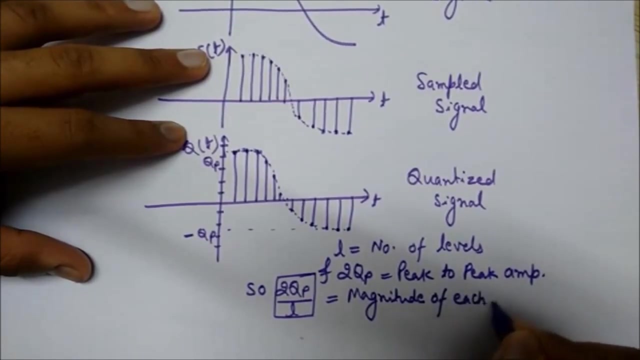 beep 2 peak amplitude. okay, let's speak to peak amplitude. and so you can say that two times of QP by L, two times of 379, 0 and sometimes L also four times QP, half struggled. your computer-board QP divided by L will be the magnitude of each level, magnitude of each level. so. 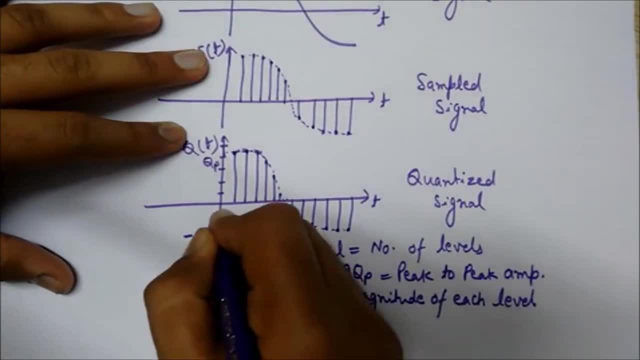 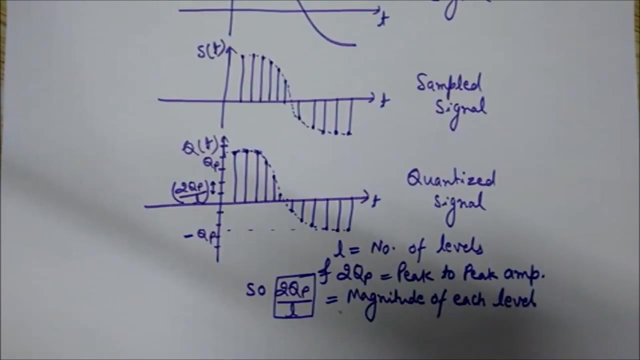 what is 2 QP by L or the magnitude of each level? this is the 2 times of QP divided by L, this distance or this distance. these all are same understanders. so it is clear that as the number of levels increases, the accuracy of the quantized signal increases. the quantized signal is just an